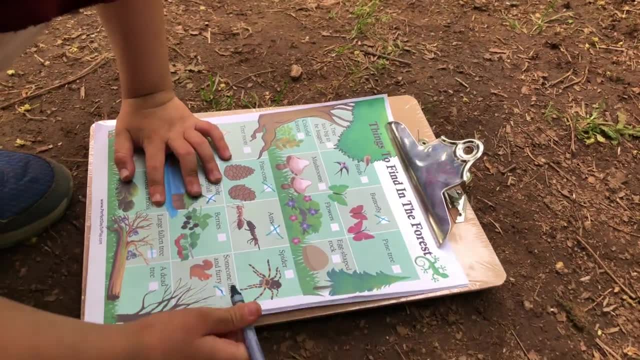 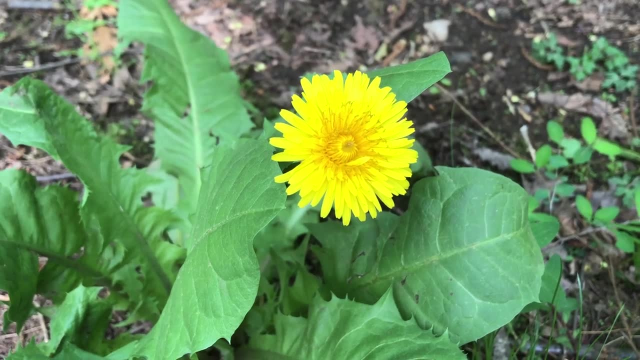 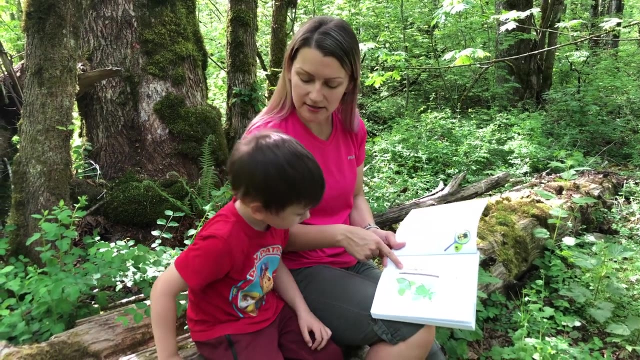 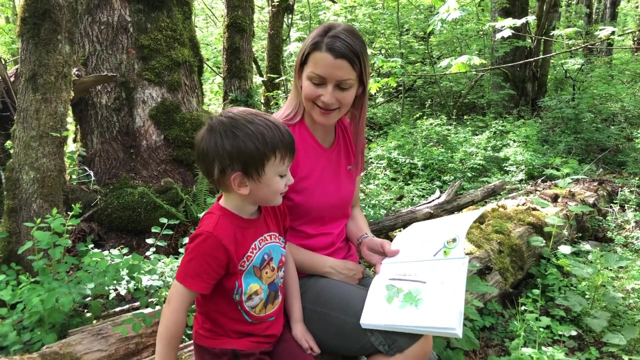 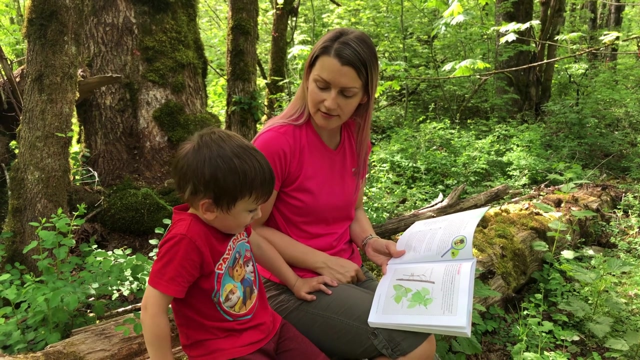 This one, Like this, Like this, And what is it that looks like a stick and crawls the tree branches, but it's not a stick. What is that? A walking stick, A walking stick. And what is it that looks like a leaf, but it's not a leaf. it crawls over the tree. 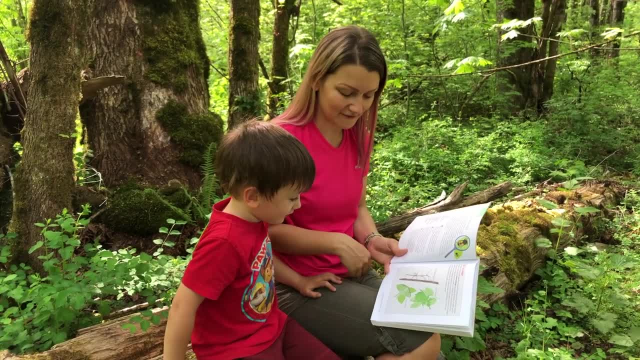 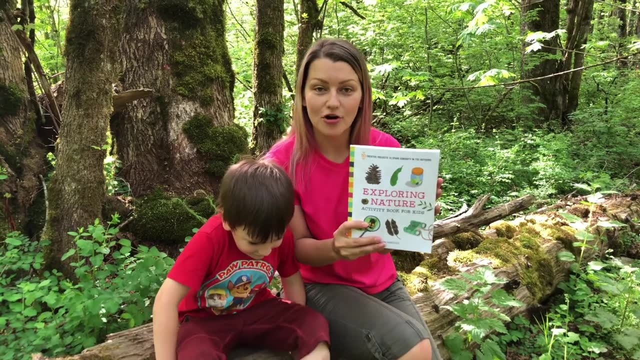 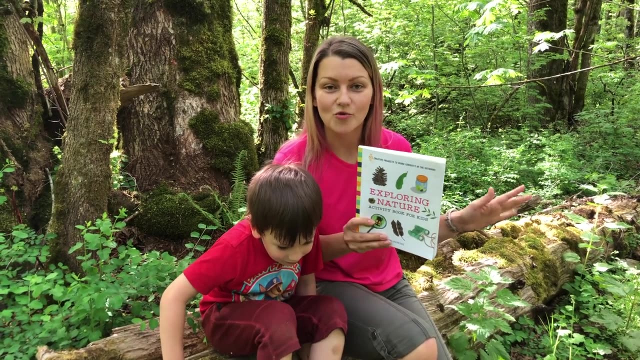 A tree, A leaf bug. Here we want to share a book with you that we really like. It is exploring nature activity book Has a lot of interesting activities which are nature related. You can use it on the trail while you are walking around and observing and learning about nature, about plants and animals and insects. 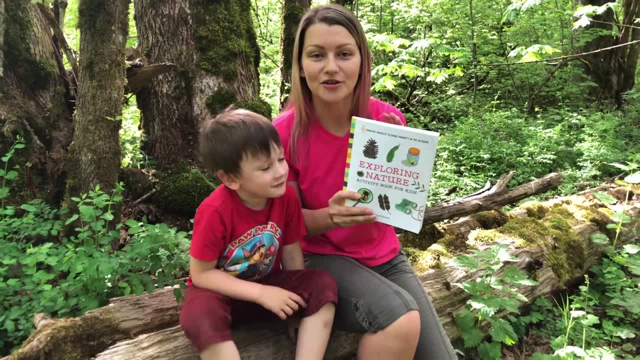 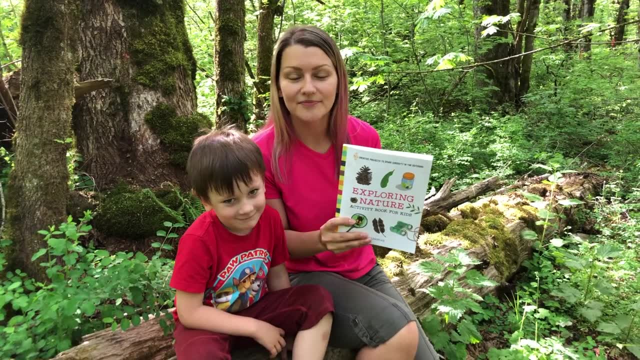 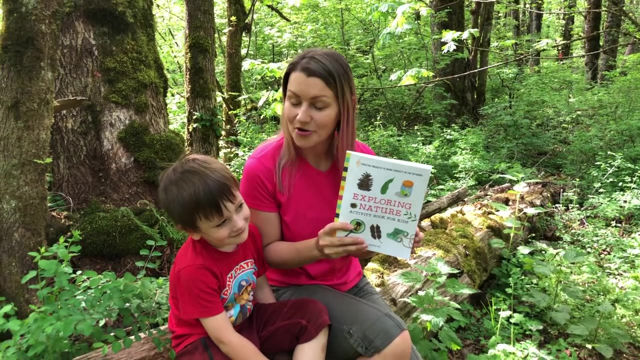 You can also use it at home when you get home, and you can make crafts after little things that you picked up along the trail. It does inspire natural curiosity, creativity, the discovery sense, and very good for younger kids who are just learning to be naturalists. 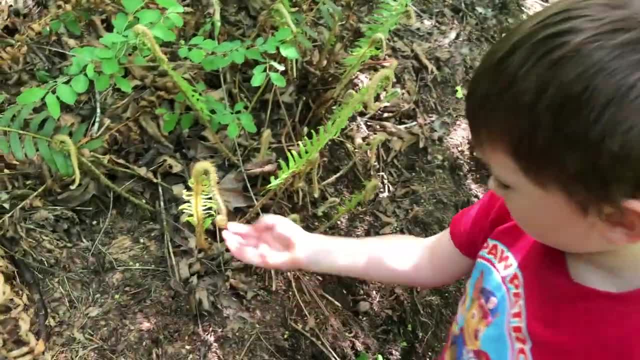 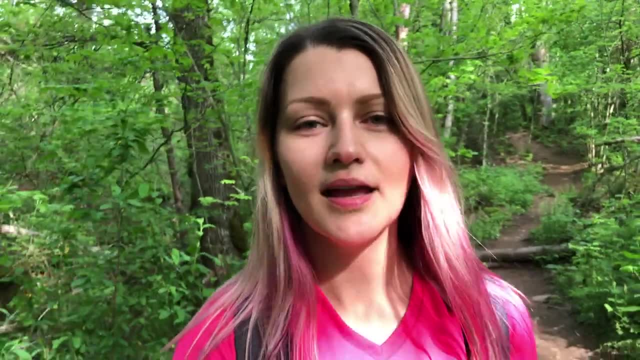 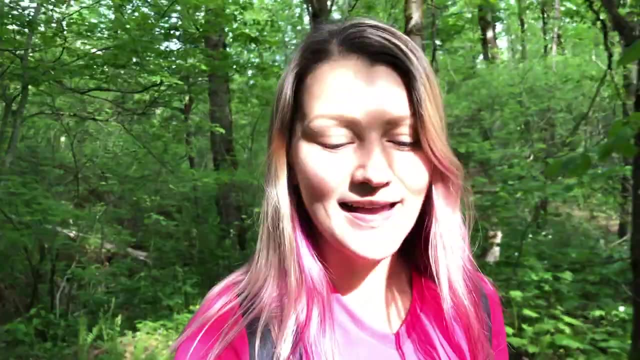 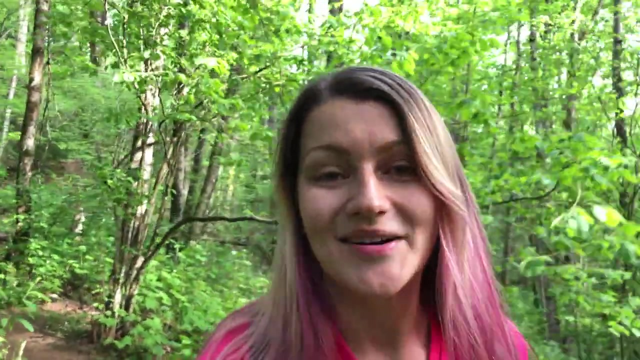 What is there? a butterfly? Yeah, a little one. A tree? An egg? The next tip is quite controversial and it is about giving your child a phone or a camera to use while they are on the trail. You can use your old phone or purchase a very cheap phone with a good camera and turn off all of the apps. 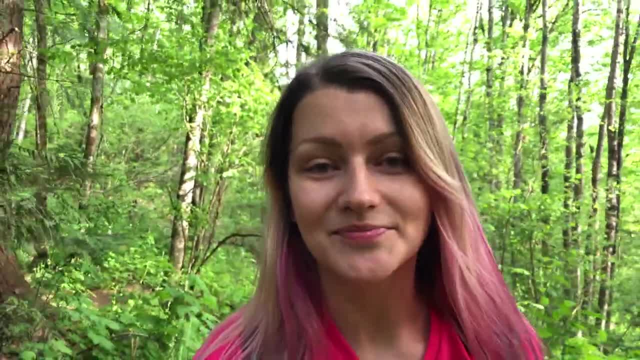 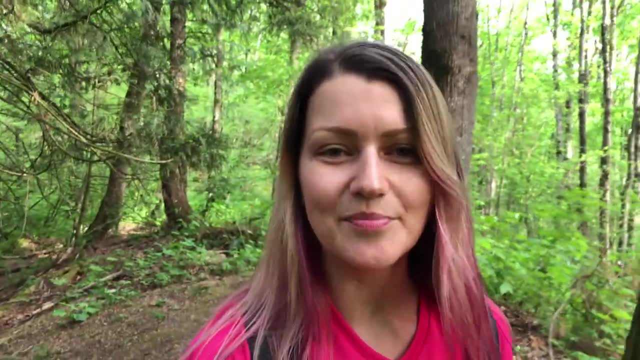 Just leave them the photo app. That's it. Because you know the kids get pretty bored when you are jumping around and taking photos of them off the beautiful landscape, You are asking them to pose for the pictures and to pose with you. 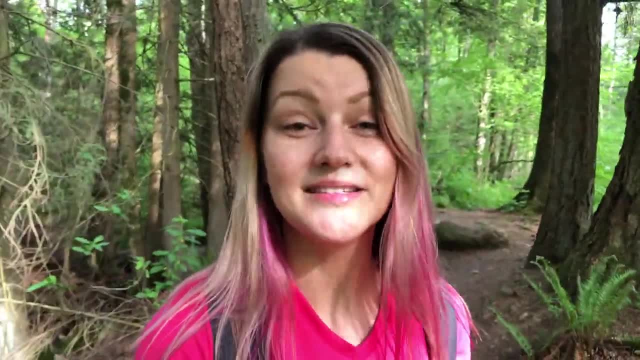 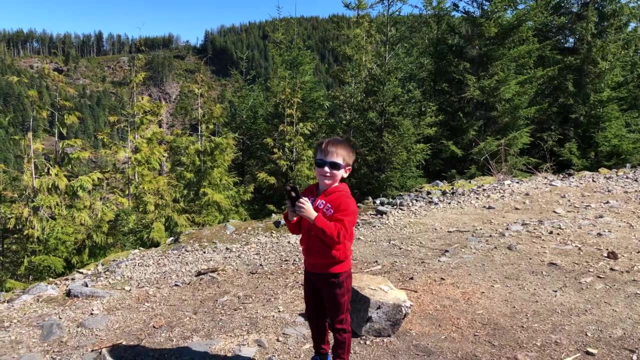 You are asking them to pose with you, But they cannot really engage, And having their own camera would give them a chance to play with you using, well, the same toy, I would say, And you know, maybe they would ask you to pose for them. 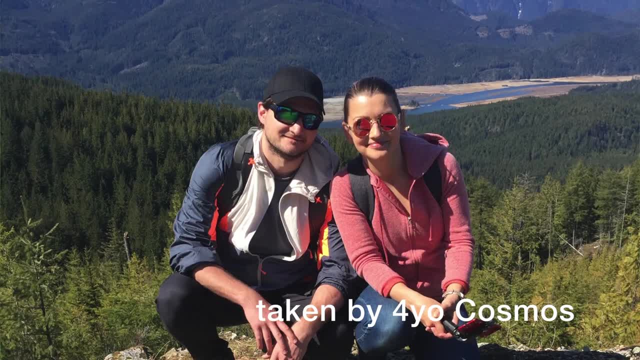 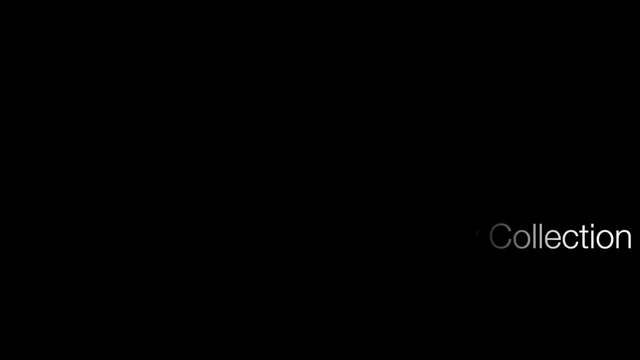 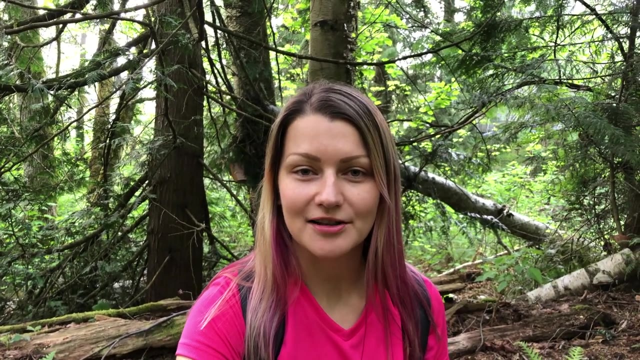 And who knows, maybe one day they would become the new landscape photography star for Instagram. You never know. A cool thing that you can do on the trail that gets kids really excited is to collect those little things along the trail that you can use for crafts at home. 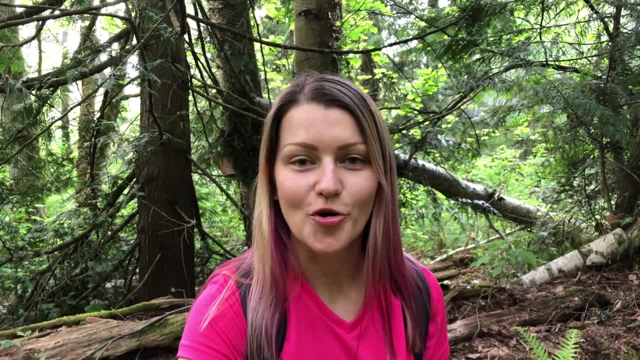 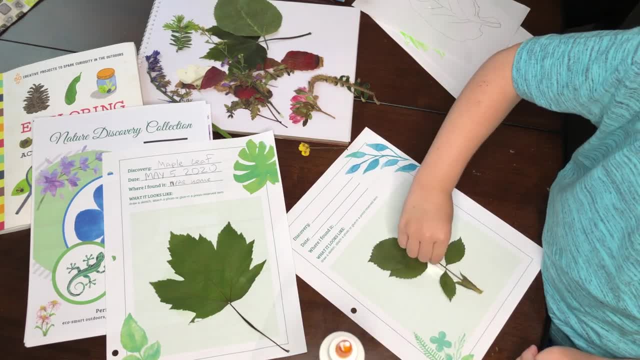 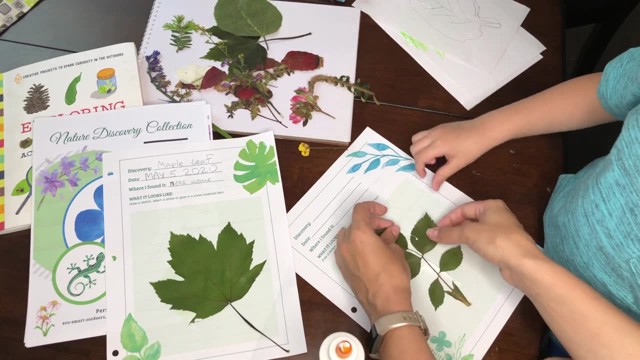 Like little pieces of wood and dried leaves and acorns and pebbles, And when you get home you can play with them, You can create crafts Or you can create your press-preserved collections. We do have printable sheets that we have developed specifically for that purpose. 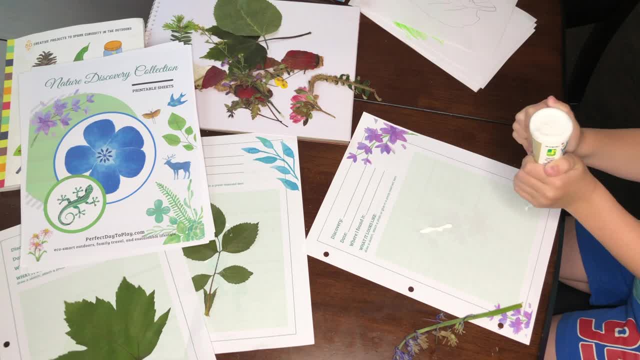 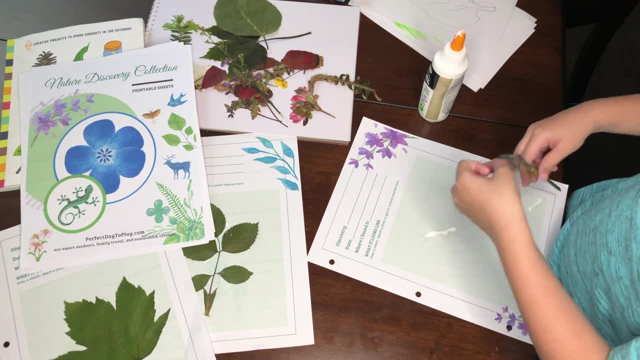 To create collections of animals and plants, just the way the real scientists do those. Those sheets can be used with a three-ring binder. Each of them has a little space where you can either stick your press-preserved plant or you can draw a sketch of an animal. 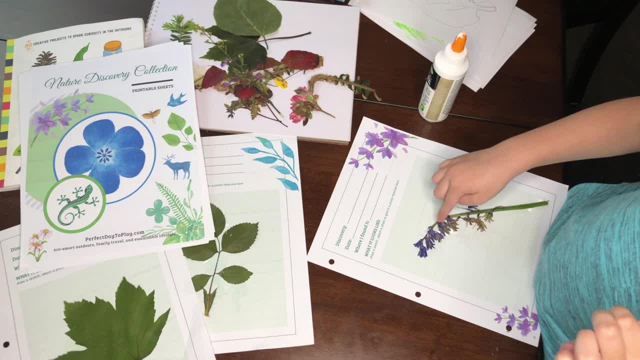 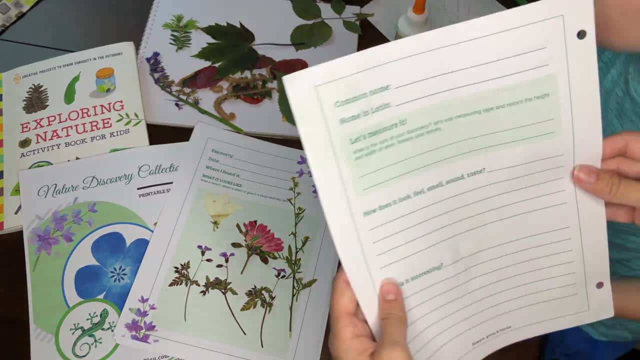 or put in your photograph that you took while on the trail. It does have a little notes area where you put in the measurements and description of your discovery, And it even has a little space where you can put the name of your discovery in Latin. 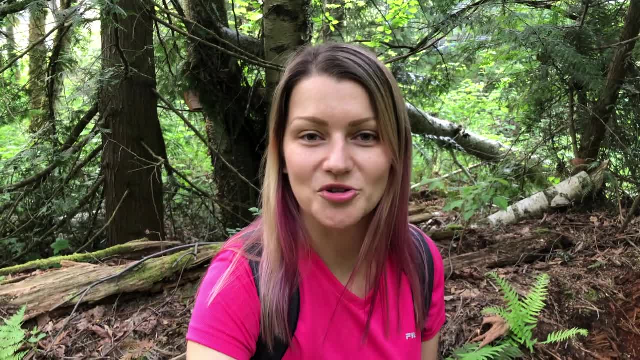 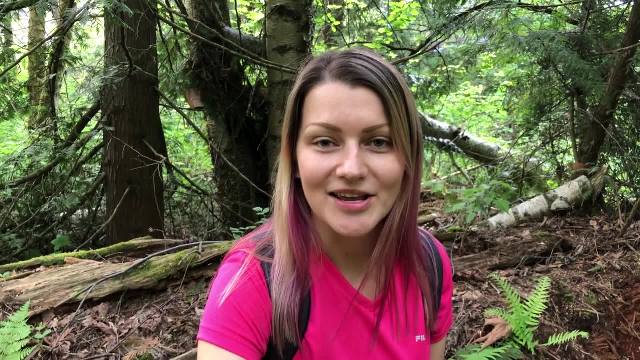 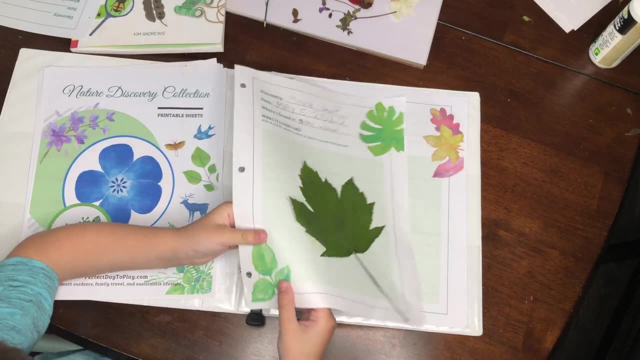 You can look up how it is called, what is the term that is used by real scientists when they are cataloguing the flora and fauna, and have that name in your collection. And the cool thing about those sheets is that you can mix and match them around. 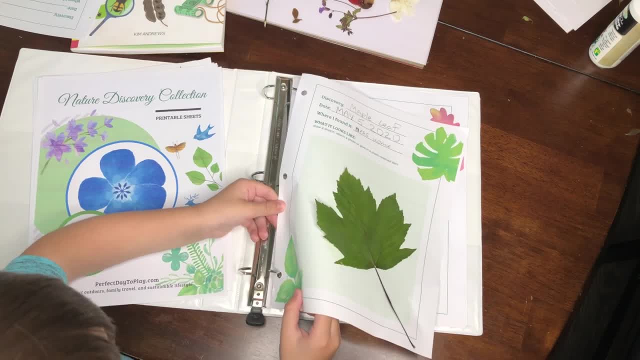 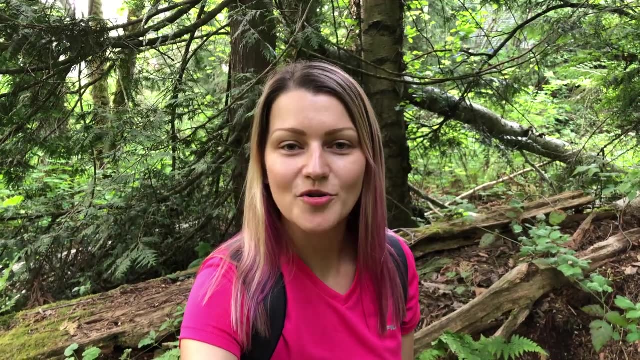 They are developed for a three-ring binder. You can easily switch or exchange your collections with your friends. I have them in 21 different templates. I am going to put a little link underneath the video where you can check it out and get those sheets for your kids. 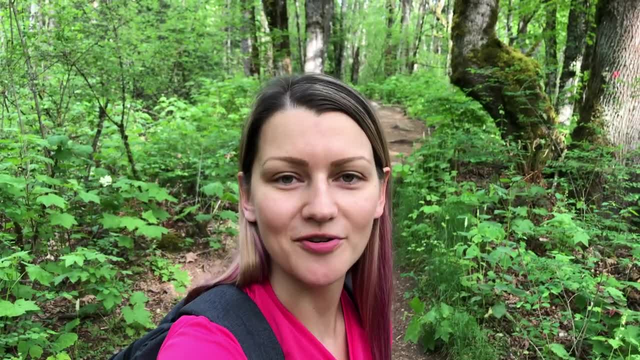 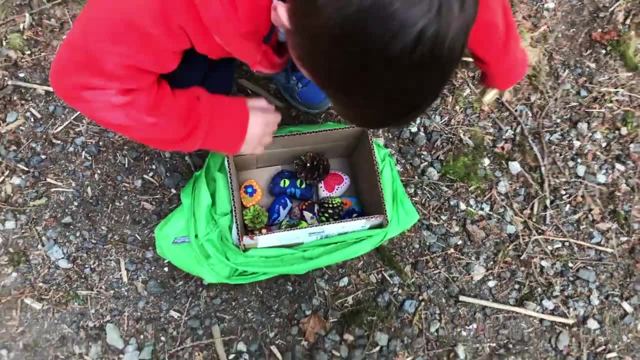 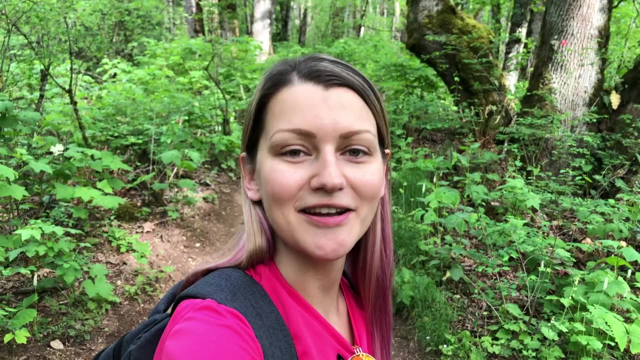 One of the other fun things that is getting really popular right now is painting rocks and hiding those rocks along the trails. You can make a fun game, a treasure hunt game, out of leaving the rocks for someone else to find, or looking for rocks, taking photos of them. 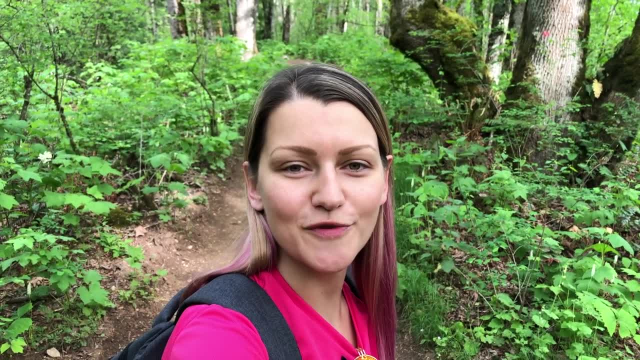 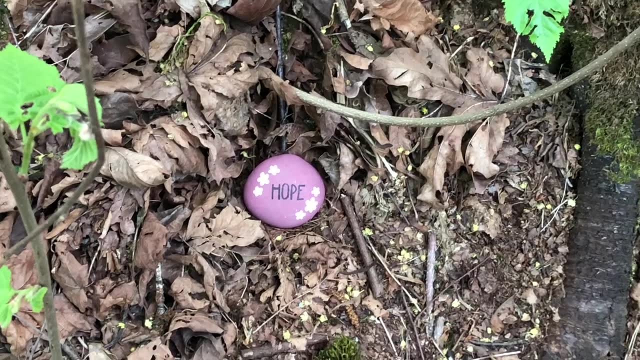 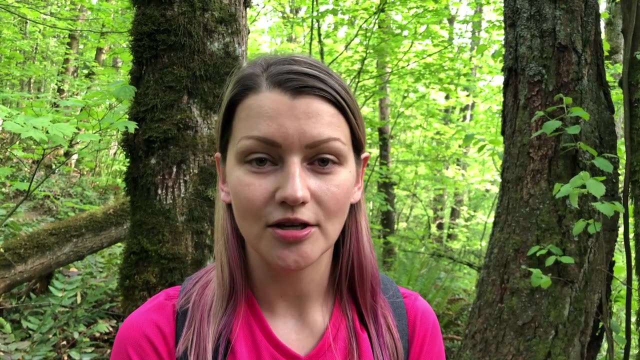 and making a collection of the rocks that you found on the trails. So your child is super eager to go on another treasure hunt as soon as possible, And we just found another rock right here. If you want your children to get interested in hiking, 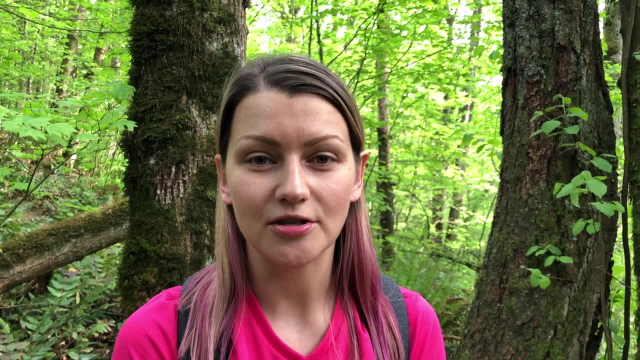 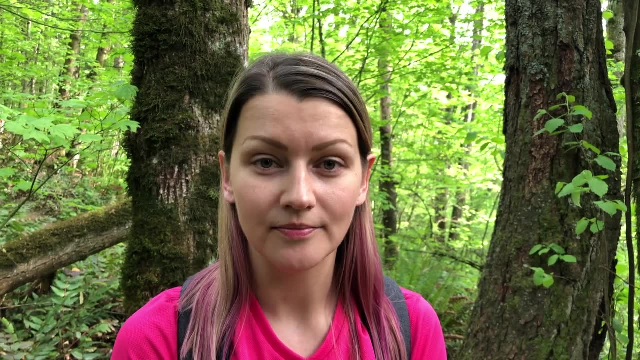 you should have safety at the top of your priority list Because if something should ever happen to them when they are on the trail, if they get injured or hurt, they would probably not want to hike with you again. I do have a blog post.